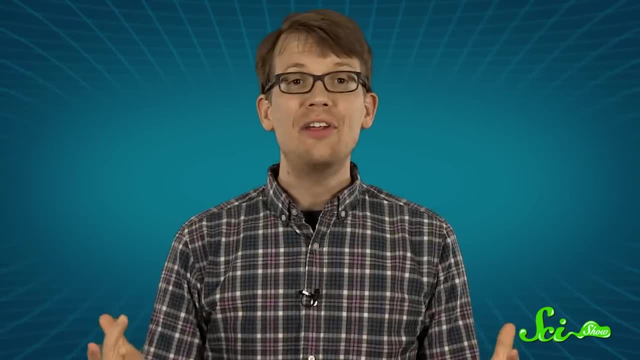 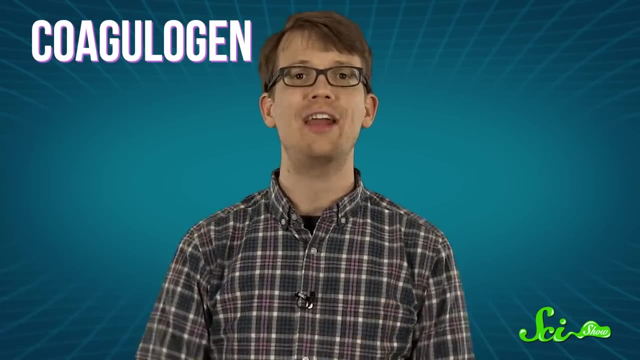 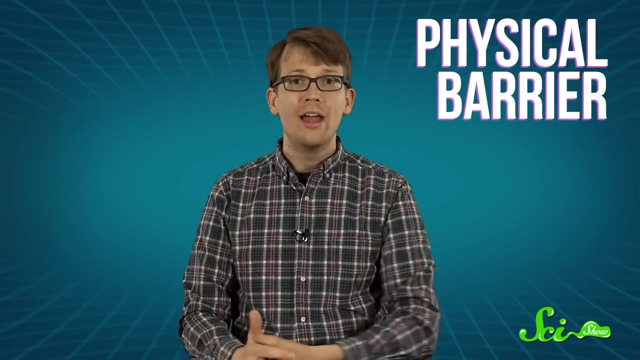 inactivates unwanted bacteria, viruses and fungi. When the blood cells sense some bad guy invaders, they release a protein called coagulogen that forms a gooey barrier around the infecting agents, preventing their spread. That clot of gooeyness actually creates a physical barrier sealing up the wound and 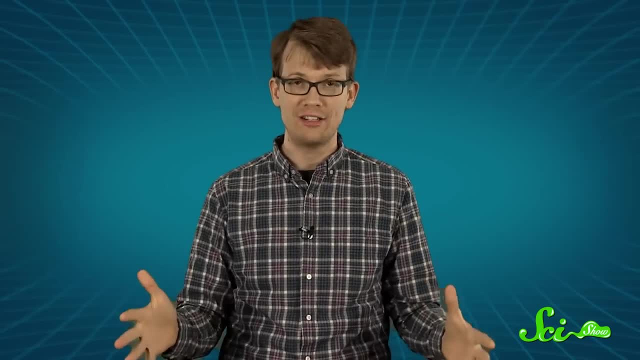 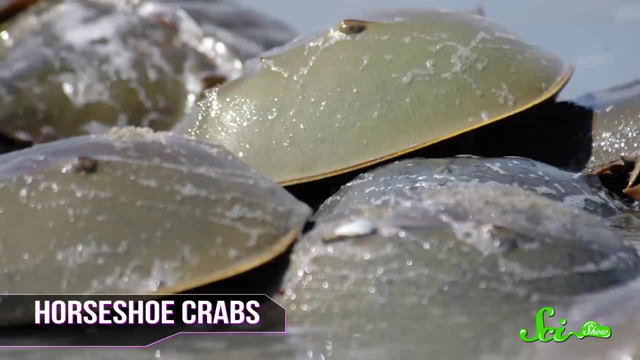 preventing further infection. It's an amazing internal defense mechanism. Humans, We have no such ability, so for the past 50 years we've been stealing it from the horseshoe crabs, Ever since American physician Frederick Bang discovered the weird power of horseshoe crab. 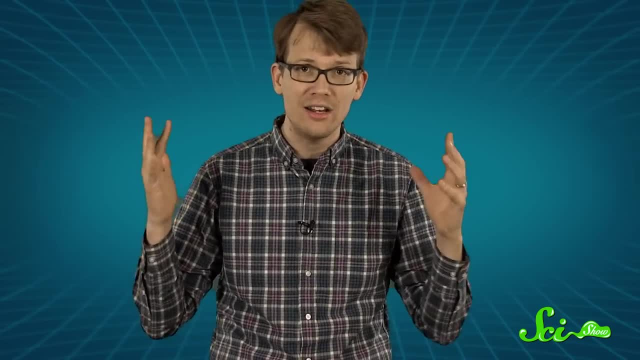 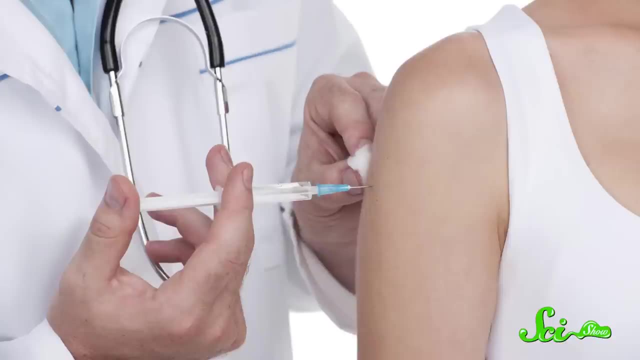 blood in the 1960s. these ancient sea creatures have played an essential yet largely unknown role in human medical treatment. If you've ever received any kind of drug or vaccine through injection, it's because these crabs made sure that that injection. 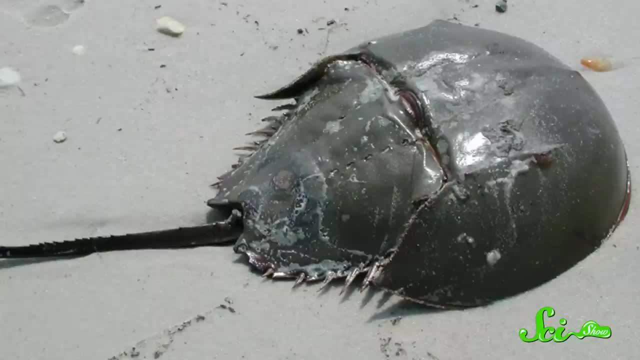 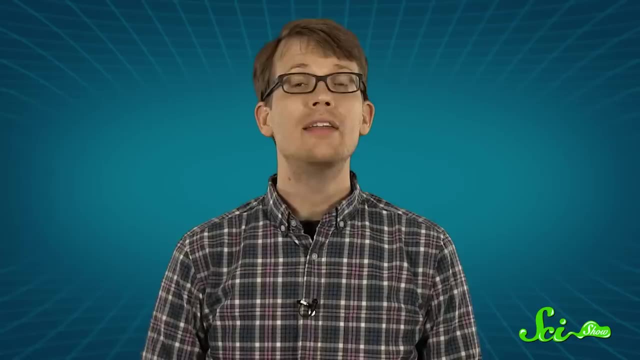 was effective, was bacteria-free. The whole thing starts when horseshoe crabs are collected from the wild, transported to one of only five production labs in the world and then rigged up for a blood drive. Needles are inserted around the heart and up to 30% of the animal's blood is removed. 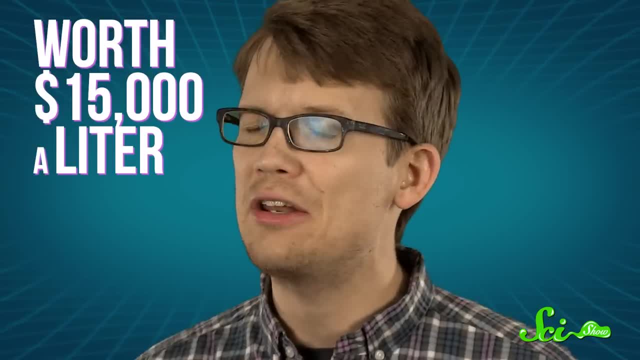 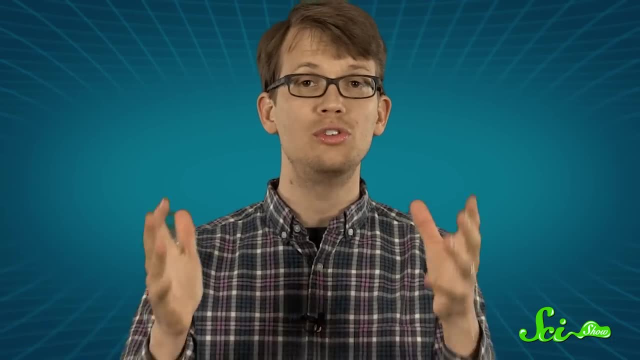 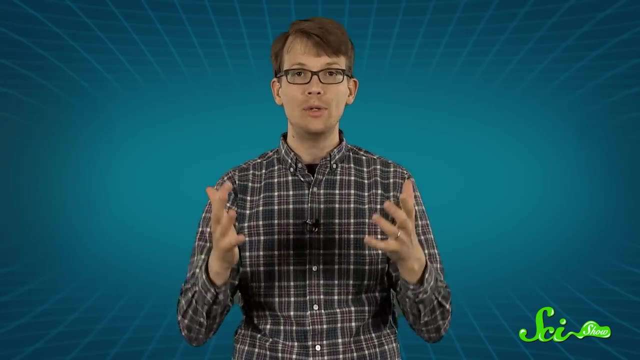 This stuff is liquid gold. It can go for $15,000 a liter From there. scientists extract the coagulogen from the blood cells and use it to test solutions that are used in injectable drugs and vaccines. If the crab blood extract finds unwanted bacteria in the solution, it immobilizes it in a gooey. 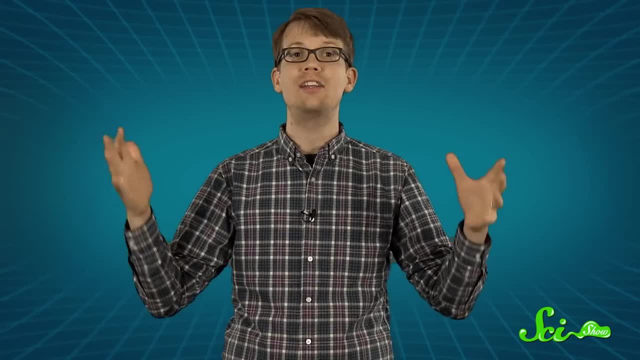 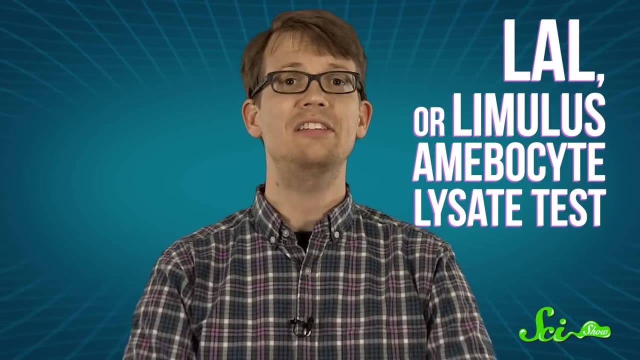 clot. So if your sample doesn't form any clots, you know that it's bacteria-free and safe for human use. This simple procedure, called the LAL or Limulus Amoebocyte Lysate Test, is nearly instantaneous and no other test works as well. As for the crabs themselves, most seem to bounce back several days after being released back into the wild, But some folks are concerned that the bloodletting weakens them more than we think, So LAL manufacturers take care of them. They tend to only collect blood once a year to ensure that they're not double-dipping. 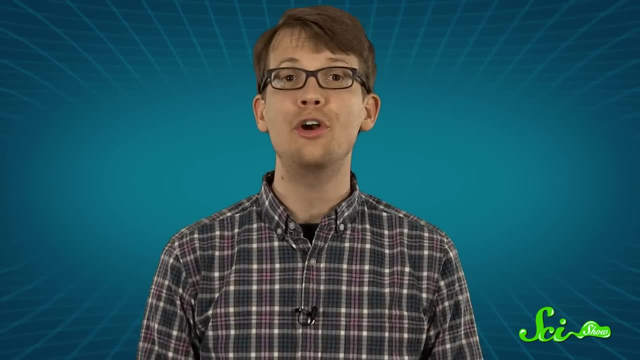 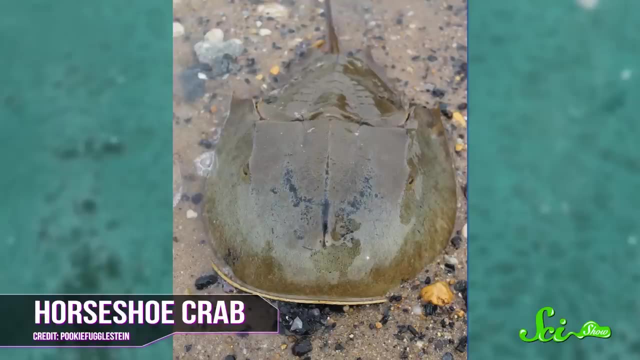 on the same crabs, and research is being done to come up with a synthetic alternative so that we can eventually leave them alone. Until then, next time you get a shot, give thanks to all those old horseshoe crabs who made your good health and your sore arm possible. 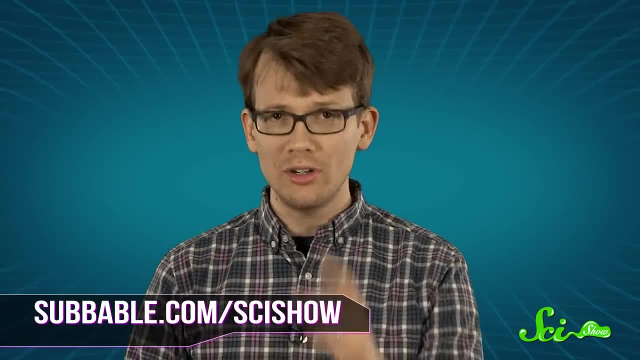 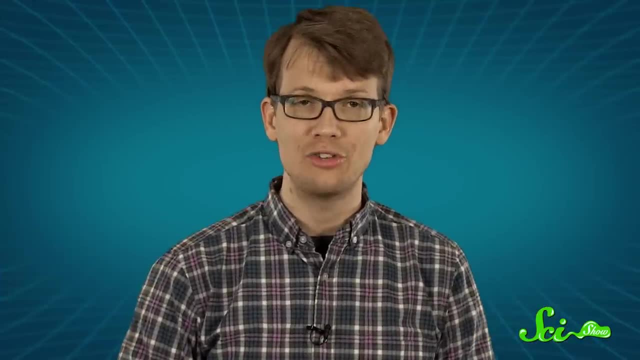 Thanks for watching the SciShow Dose, especially to our Subbable subscribers. To learn how you can help us keep sharing wonderful science like this, just go to subbablecom. And don't forget to go to youtubecom. slash scishow and subscribe. 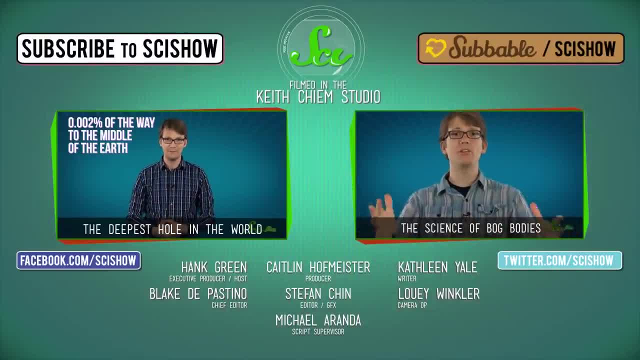 We'll see you next time. Bye, Bye, Bye, Bye.